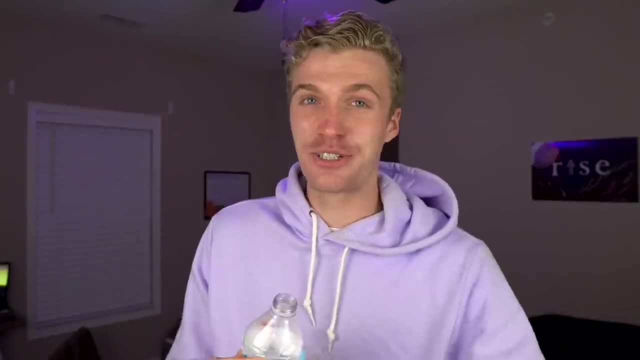 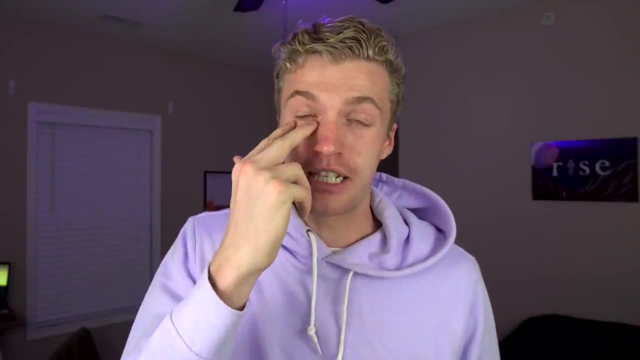 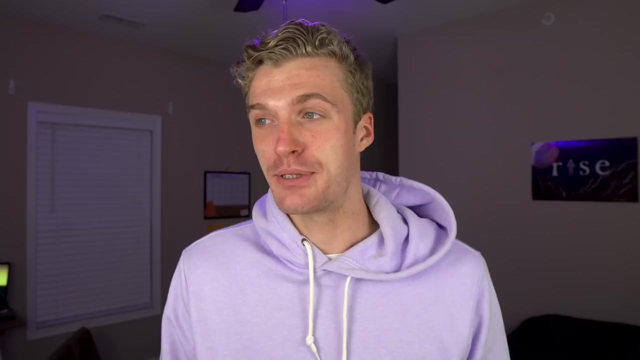 with target practice, but do not shoot these at people. I, true story, have been on the wrong end of one of these and my eye was actually bleeding. My eye socket was gushing blood. This was back in high school. My friend, Mike Kramer, shout out. Mike shot me in the face with one of those caps. 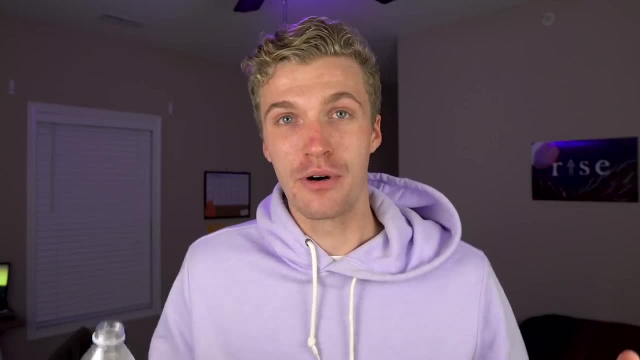 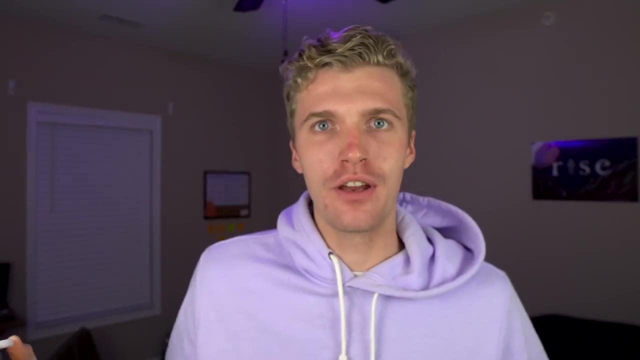 and it nearly made me blind in one eye. So do not do that to anyone And I do not endorse it. So, number two: once that cap got shot off like a cannon, what are you going to do with it? Can you still have fun with it? Yes, of course. What you're going to do with this cap? 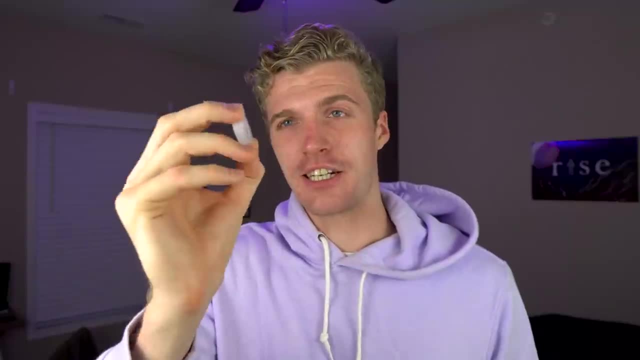 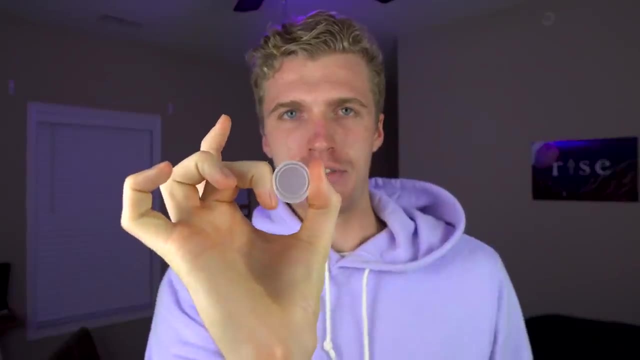 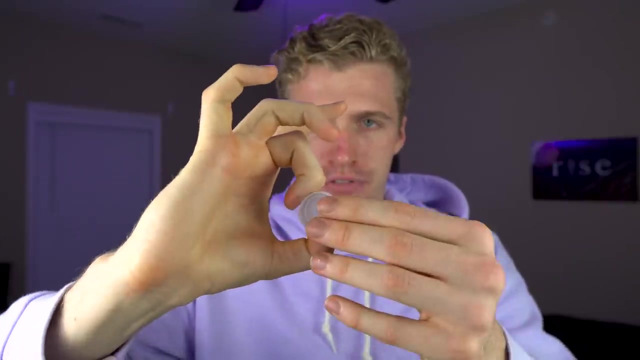 is: you can throw it almost like a Frisbee with this disc-like shape, And the way you're going to throw it is with your middle finger and thumb. The cap goes right in this little crevice like that. So that is the grip you're holding the cap in And what's going to happen is your middle. 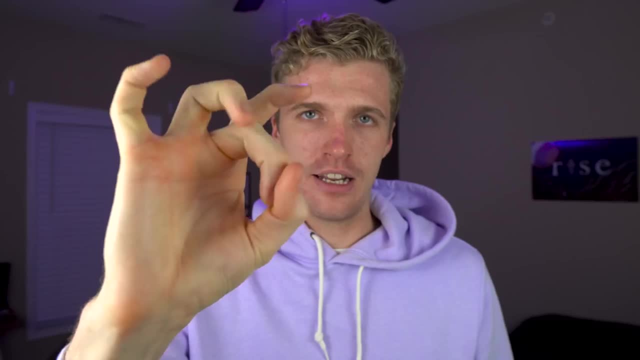 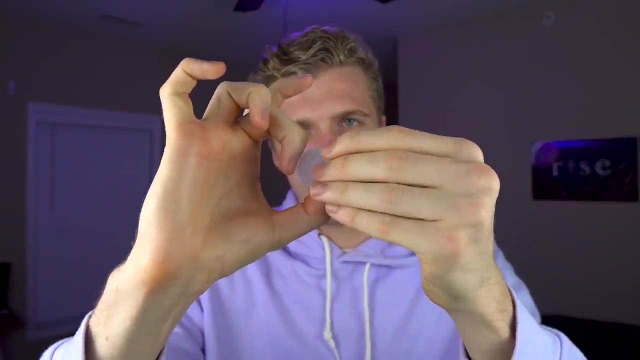 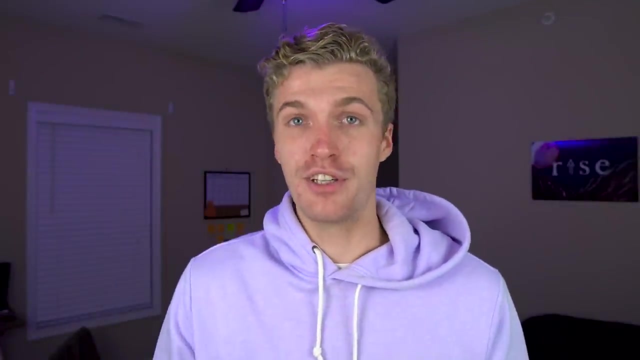 finger is going to shoot in towards your thumb like that and kind of flick out And what's going to happen is the cap is going to rotate forwards like that off of your middle finger And it's really just going to shoot and rotate through the air really fast If you get your arm involved into. 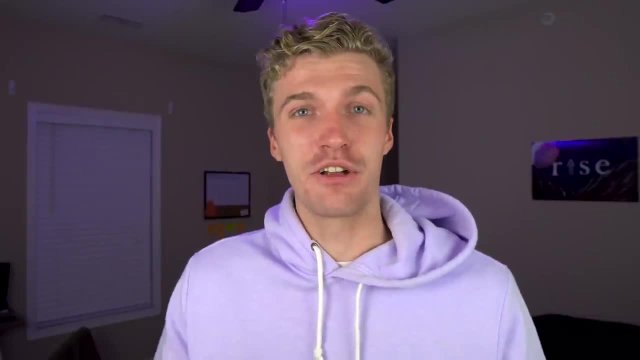 it. you can fling these things hundreds of yards. It's really fun. I would highly recommend you try it. Super easy And, by the way, if you have a Gatorade cap, like those big fat Gatorade caps- 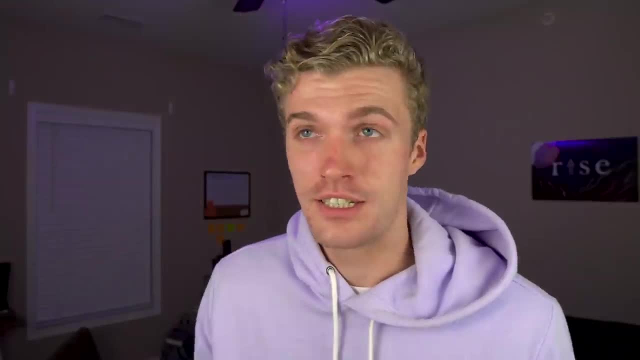 you can zing those like hundreds of yards with just that. So if you have a Gatorade cap you can. a little bit of practice. Something I used to do with my friends back in middle school is we'd play like laser tag, but with the caps You just boom, boom, shoot each other with them. A little less. 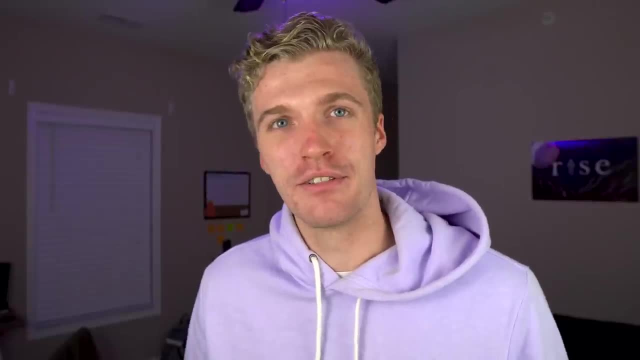 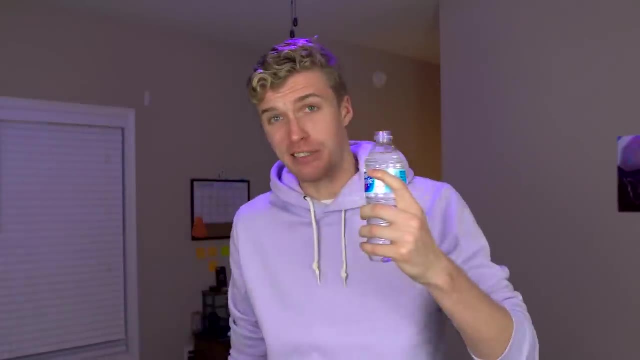 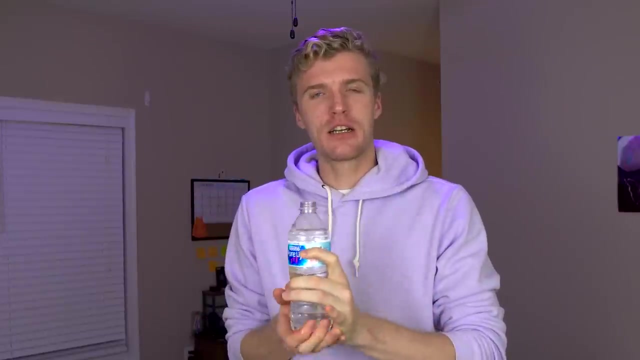 dangerous than you know. the rocket on the first one, Not as fast, but just as fun. So number three, your magic trick. All you need is a semi-full bottle of water, So maybe take a swig so people know it's real. Now, for that you don't need the cap, because this is all about water pressure. 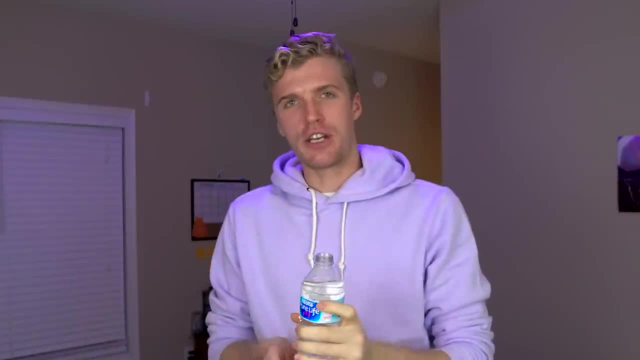 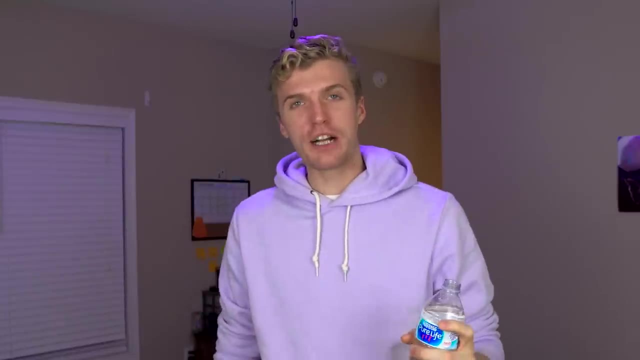 right The suction you can get with your hand. So all you need to do right is you can seal the vacuum pressure inside the water and make the water no longer be affected by gravity. Here we go. This could get messy. 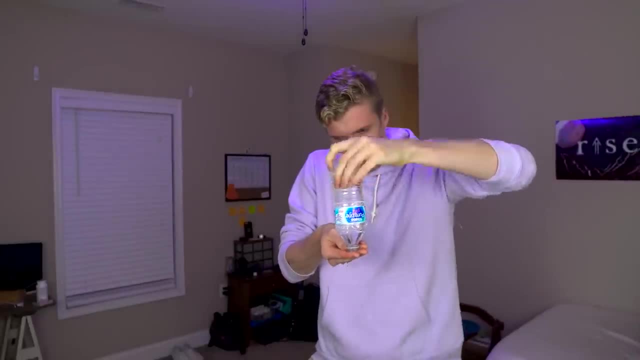 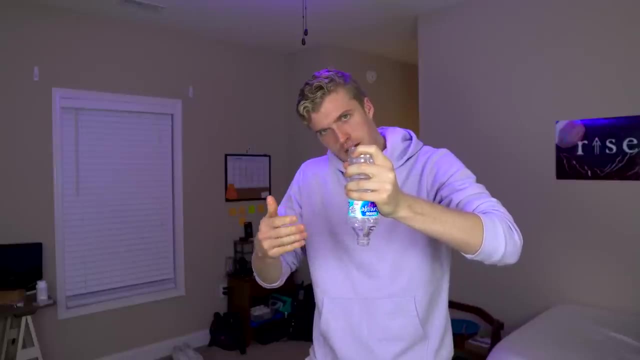 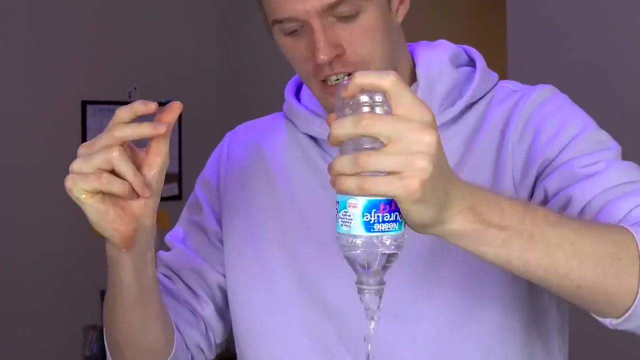 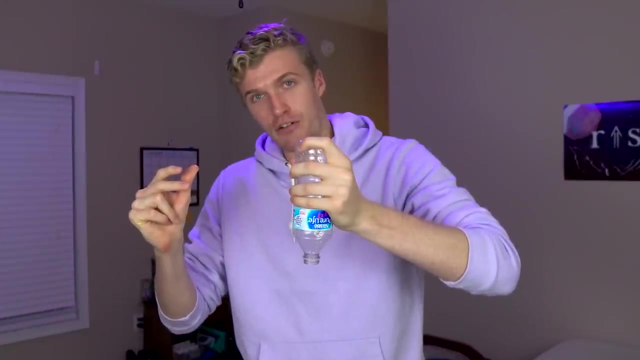 I spilt a little bit, but now my hand has it sealed And, just like that, the water is no longer affected by gravity until, guess what, I snap my fingers And it pours out all over my bedroom floor. Nice, The best part about this trick for me. 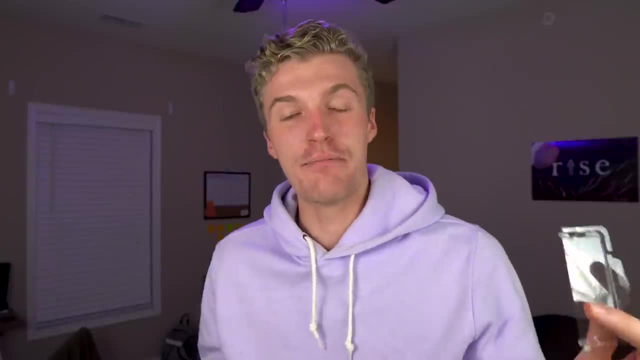 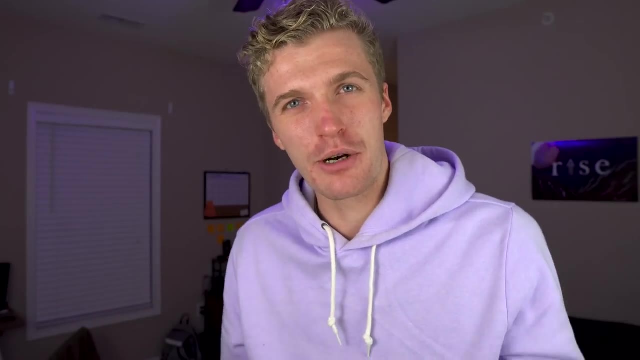 is having other people try it, because there is obviously a magical secret behind it. You're going to want to take some clear plastic, like the stuff that comes in any you know that really annoying stuff that comes in all your packages, that hard plastic. 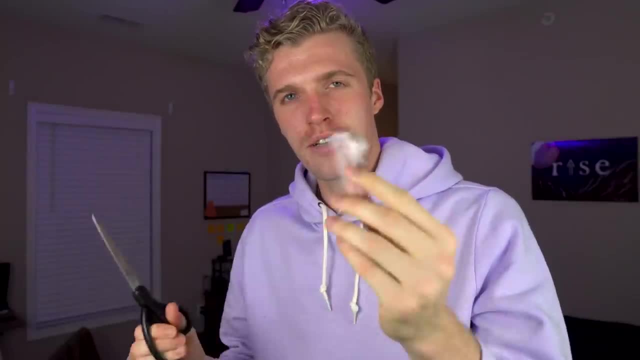 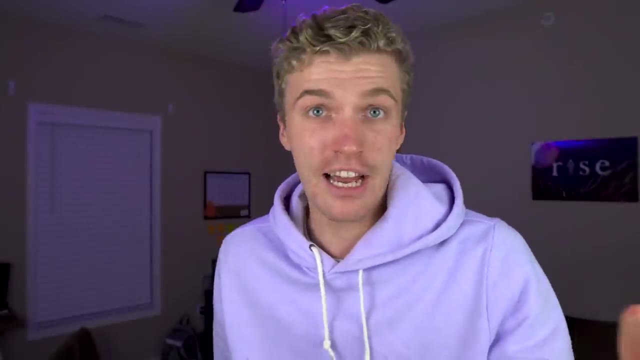 You're going to want to cut a circle, the shape of the cap. This is what mine looks like right here. Now you could put these in your wallet or something like that. have five of them on you at all times. I'll show you, guys, the exposed view right here. 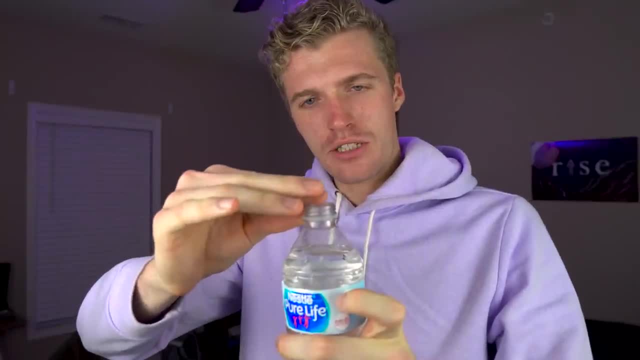 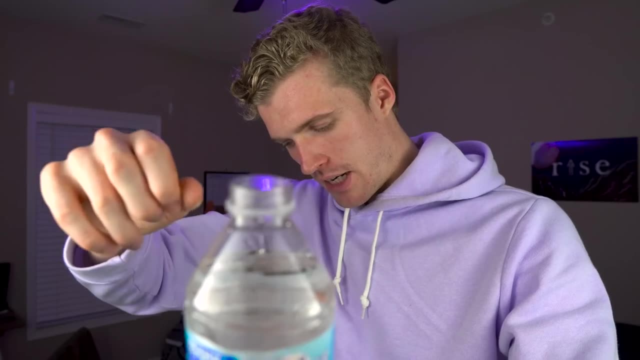 You have your little plastic piece. Basically you want to place it on top of the water bottle, just like that, So you can kind of see it right there. Mine's a little bit bigger than it should be, but that's fine, No one will notice, right? So you put it on top and then. 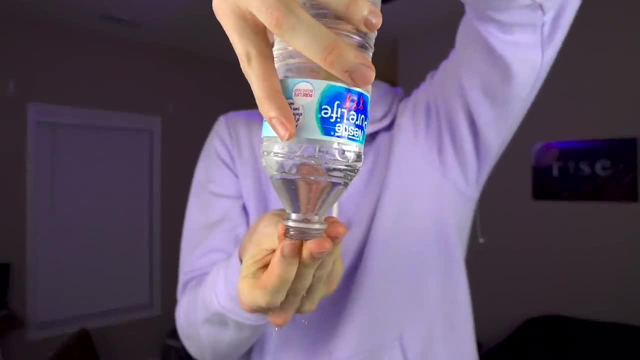 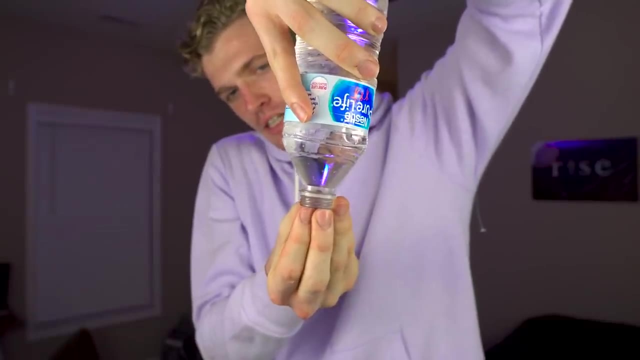 flip over And then, once you flip it over, you're going to want to put it on top of the water bottle. This is something you have to practice over the sink. I promise: Practice over the sink, because once you, you can't line it up like how I am right now, because that's too obvious. 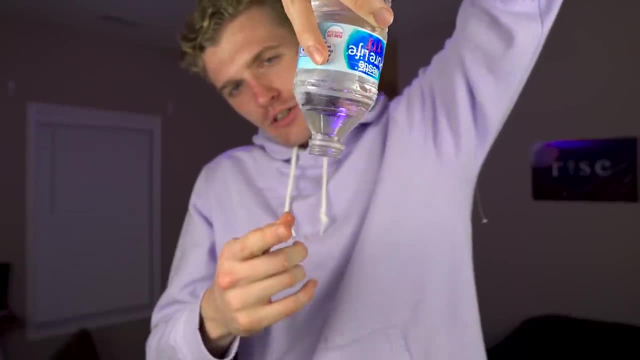 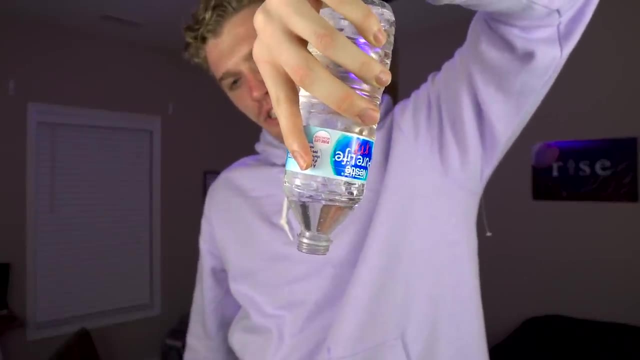 But once you have it lined up, you're going to see I'll try and tilt it up, but it might break it. You'll see the little piece of plastic on there And to let it go you can shake it or give a little bit of a squeeze while you're shaking it. 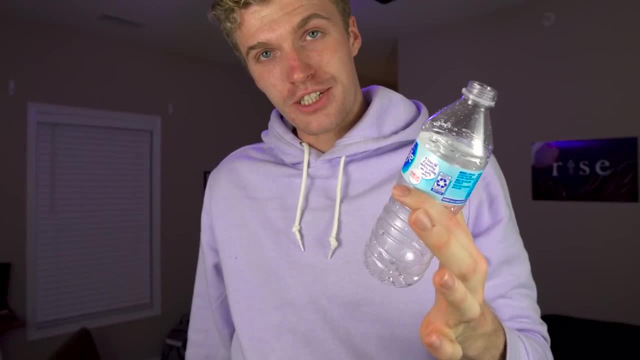 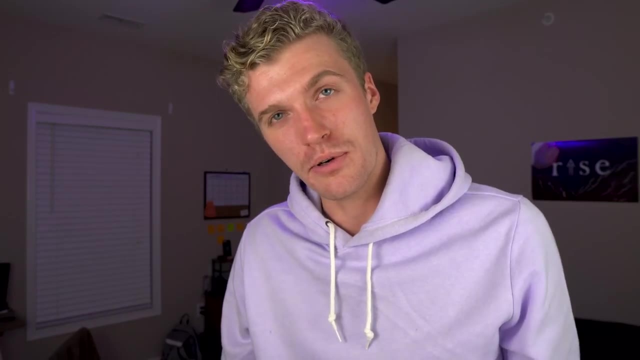 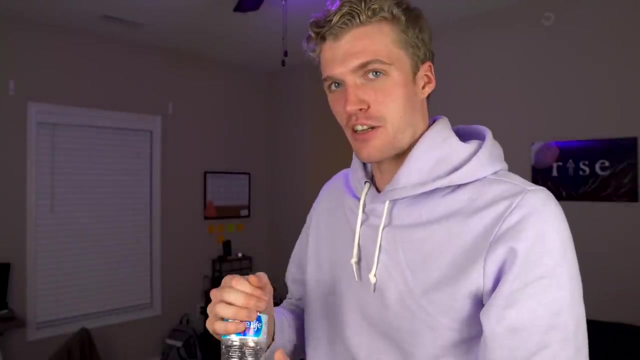 And it'll go out just like that. Number four. I don't know if everyone already knows this, but if you don't know it already, this can really annoy people, which is a good thing and a bad thing. Basically, you can make very loud noise with water bottles. All it takes is a little hit. 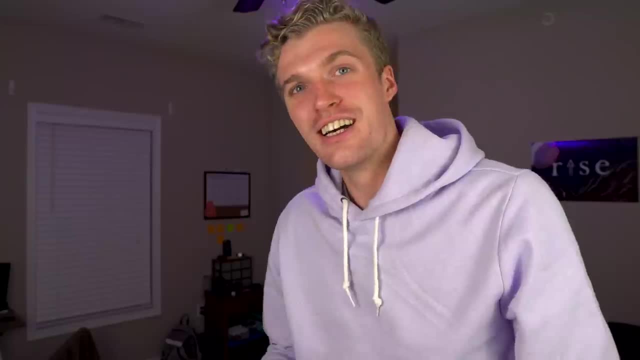 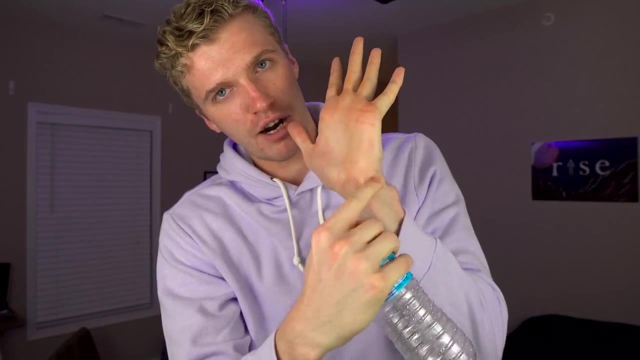 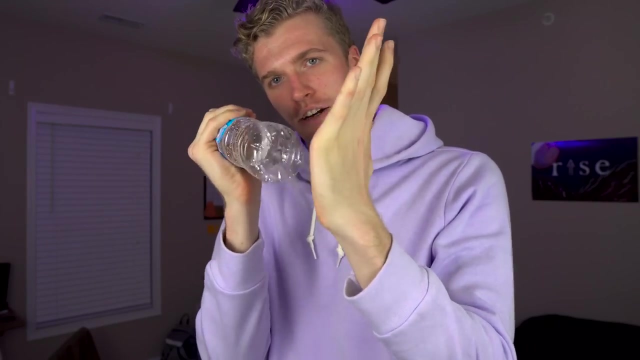 And it's almost sounds like a gunshot, Like it's so loud. This is the simplest one in all of this right. Hold it up top like that grip right there. You're going to take this part of your hand, kind of like the right palm area, this little pad right here, And you hit the side of this When you hit. 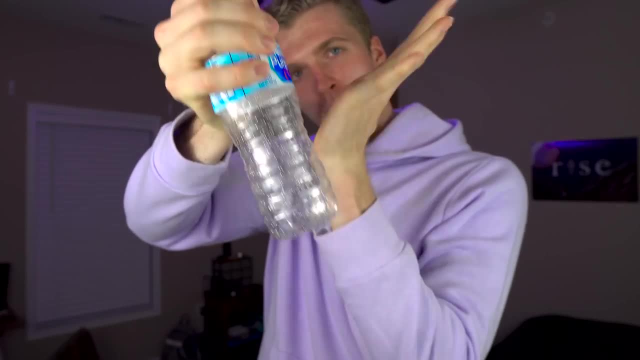 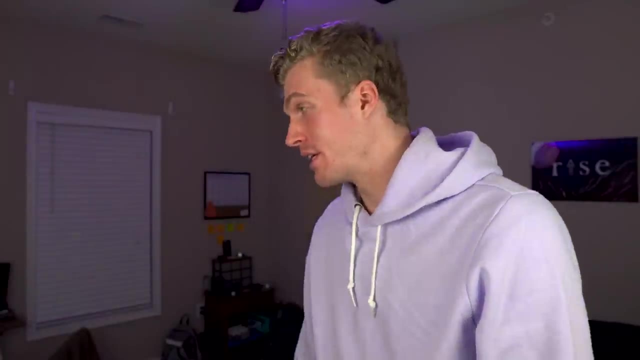 the side. what happens is it goes up And then, when it pops back, that's that noise you're hearing And it is loud. You can scare the crap out of people with this. You could use it at sporting events to distract someone where they're taking their free throws, Like: see Shaq over there. 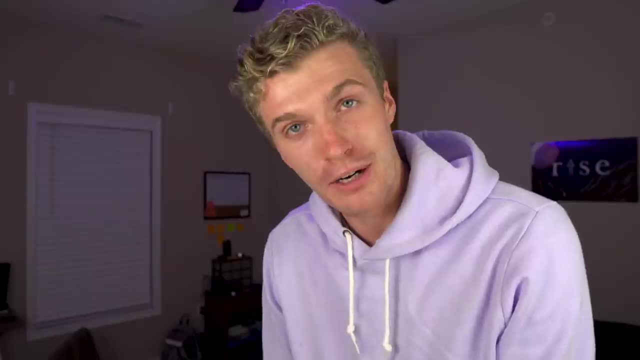 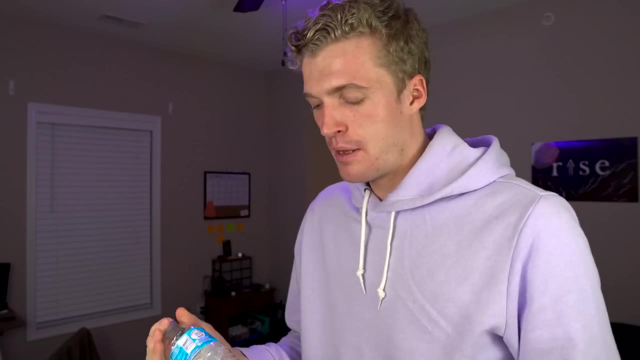 And he missed. It's that easy. Probably just broke my microphone too. You could also use it to scare people. I mean, get creative, but that's kind of a stupid one. But man, take a water bottle and try it. 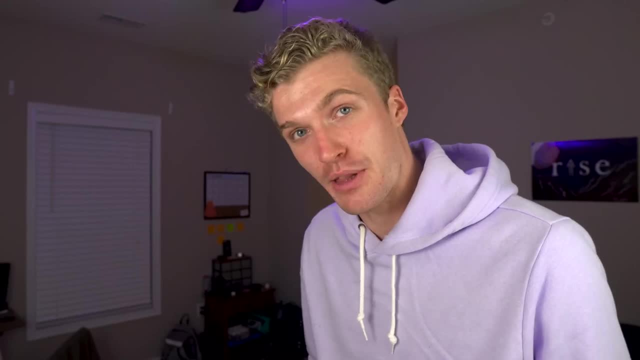 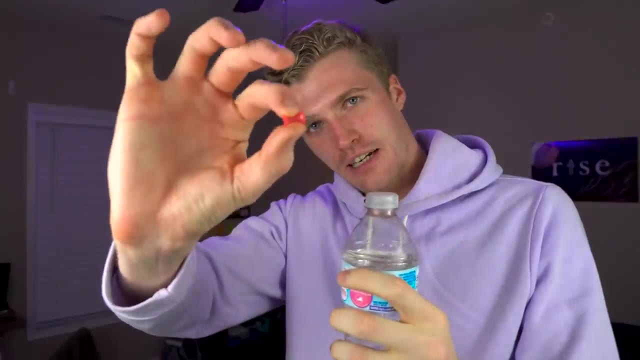 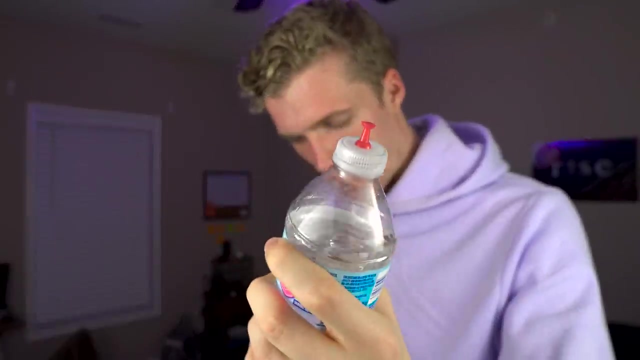 yourself, because I guarantee you the microphone is not picking up just how loud it is. Lastly, this is my absolute favorite from elementary school: You have your water bottle, Take a thumb tack like that, Go into the cap and poke a hole right in the center, just like that. Now, once you 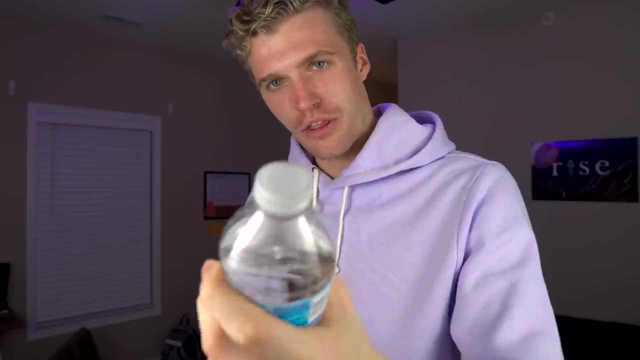 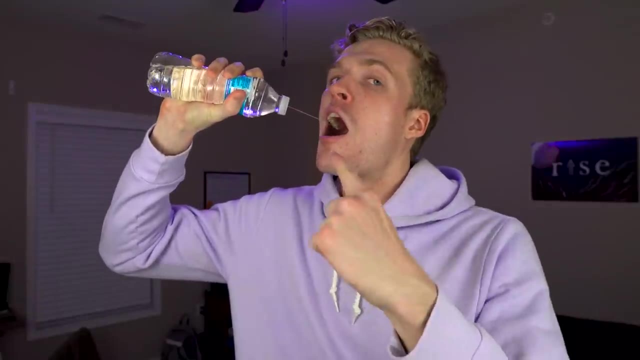 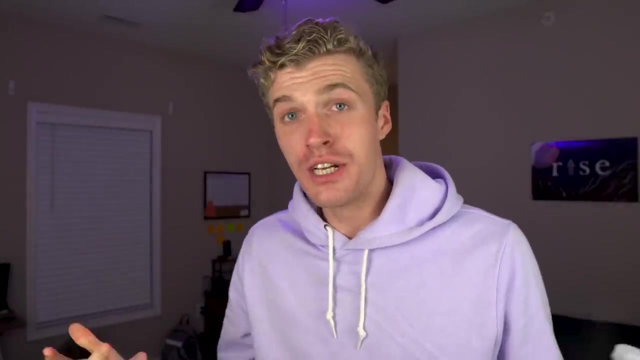 have that hole. What happens is you have that tiny hole in the thing and you have your own mini water gun. Now you can use it for beneficial things like hydrating, Get that little dose of water without overdoing yourself outside going for a run. 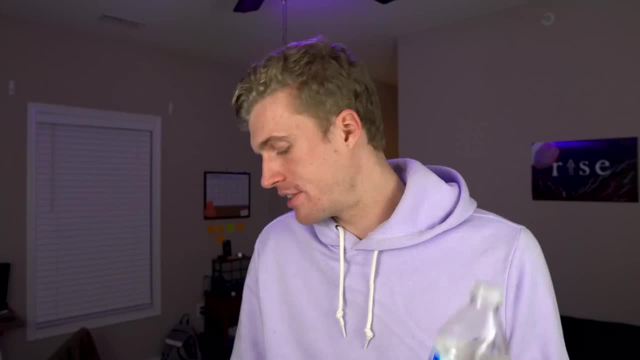 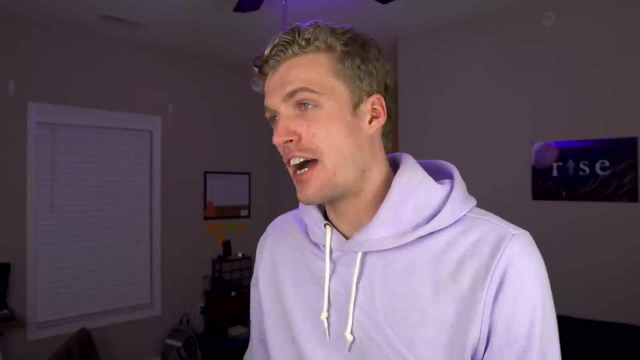 That little stream of water. you can modify any water bottle into this. You could take the tack, make the hole bigger so there's more of a stream, Or you could use it as a concealed water gun. In fact, I wouldn't recommend this, but I remember in elementary school doing this to my teacher. 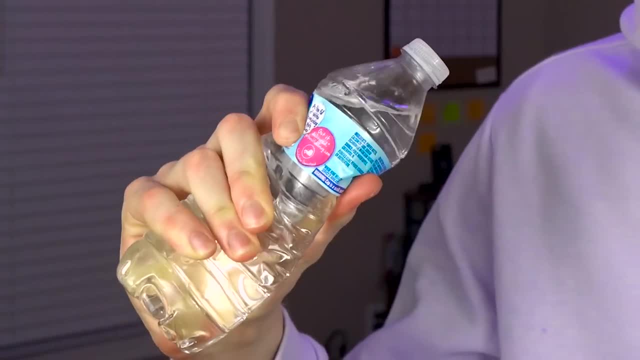 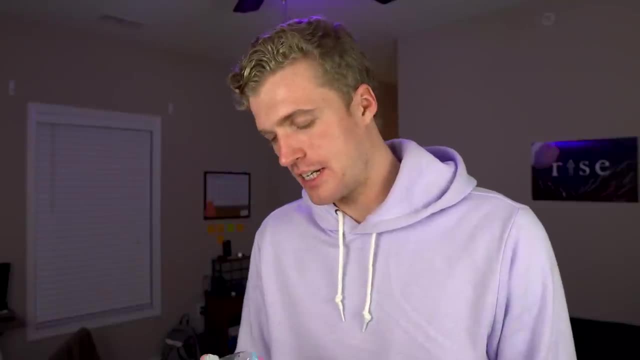 because I was a juvenile delinquent and I would. But I'd go up to my teacher and take them a second to realize what's going on. All right, well, that's how I'm going to end it. guys, That's just a beneficial one you could use. 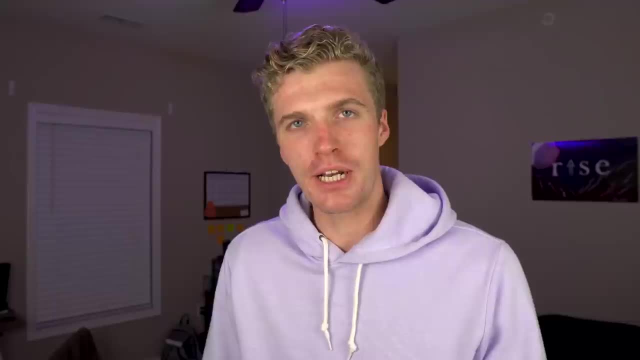 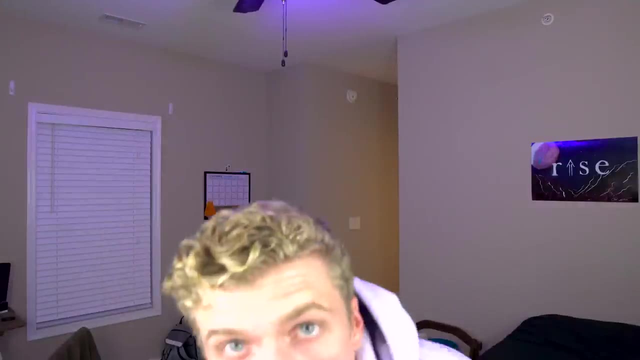 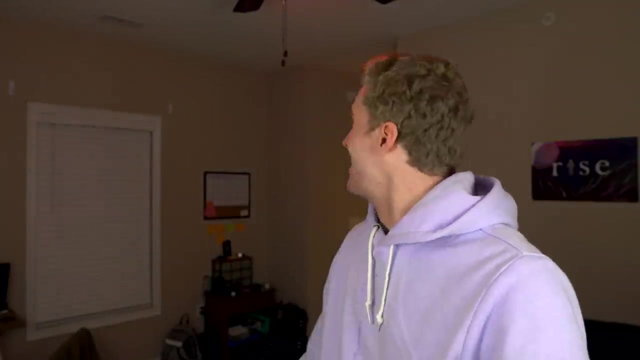 in your everyday life to stay hydrated- Very important to stay hydrated. Make sure your urine is crystal clear, Very important. Now, if you're your Alexa, turn the bedroom lights to red. Okay, 15 bucks, Little things, little things, Those aren't 15.. Anyway, if you like this type of 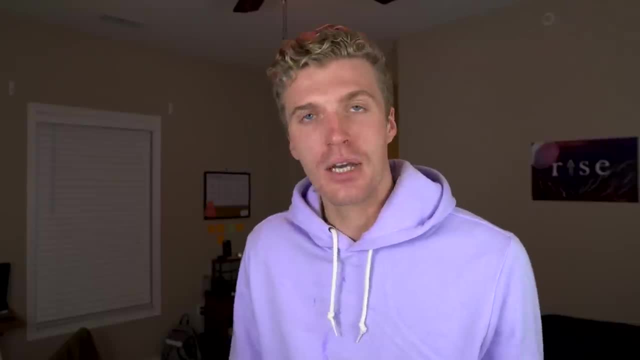 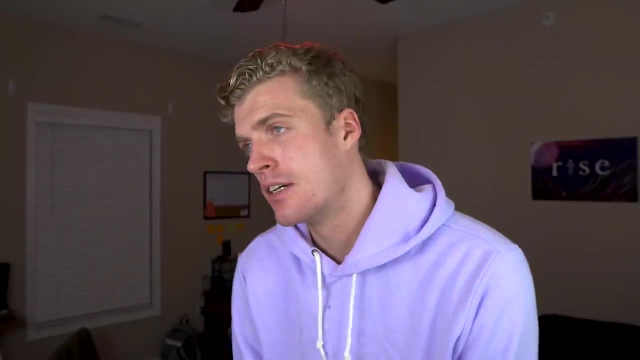 content, be sure to like. if you like the video, Let's be honest, you probably did. If not, you know you could still like it and just be encouraging. Yeah, so those are my five little tricks. Put them to good use. Don't get in trouble in school. If you do, be sure to tell.